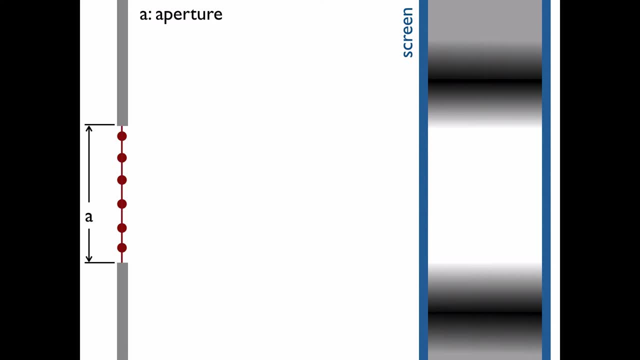 picked six of them And I'm going to look at the light pattern, not going to the middle because that's just flooding through the opening, but the first fringe, which is actually dark. So all these little spots are going to send light wavelets to the dark fringe And they're 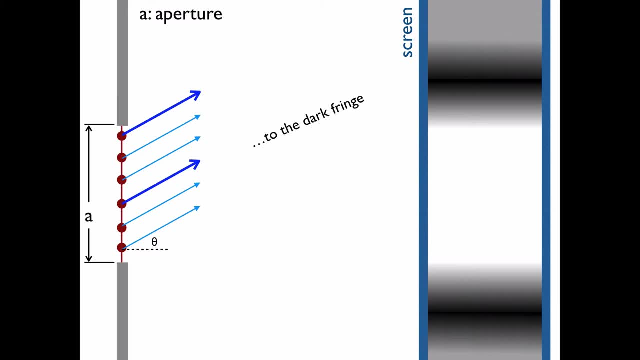 going to be at some angle theta when they do this. Now, to analyze this, I'm going to look at the top little particle and one in the middle. That's going to be half the aperture away. So whatever the aperture is, it's half way. 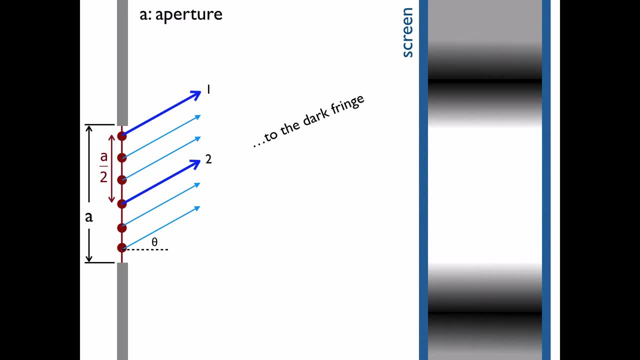 away. So I've identified these as ray 1 and ray 2.. Well, ray 2 is going to travel farther to reach that top dark spot and it's going to do by this amount. that's black. So that's going to be the path difference. That means I can make a right triangle and use a over. 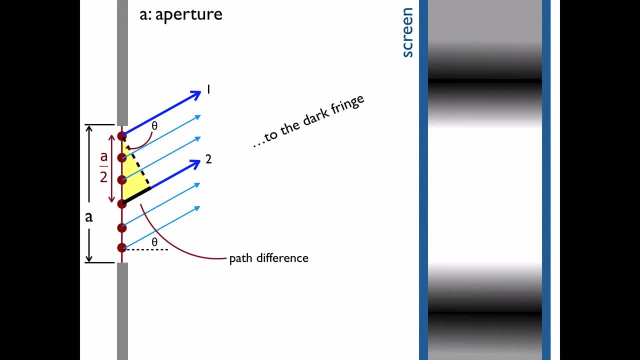 2 as the hypotenuse and I have theta and then I can find out the length. that is the path difference And that's important. I know that for constructive and destructive interference. So for this path difference, since it leads to the destructive part, it's going to be half. 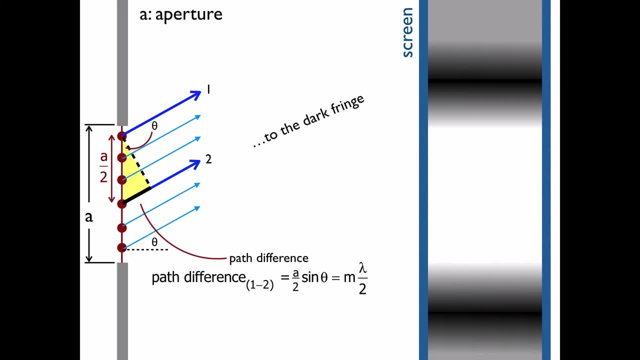 a wavelength off. So the hypotenuse a over 2, the aperture over 2 times sine theta is equal to m lambda over 2.. Well, the 2's go away, so this becomes a sine theta is equal to m lambda for dark fringes. 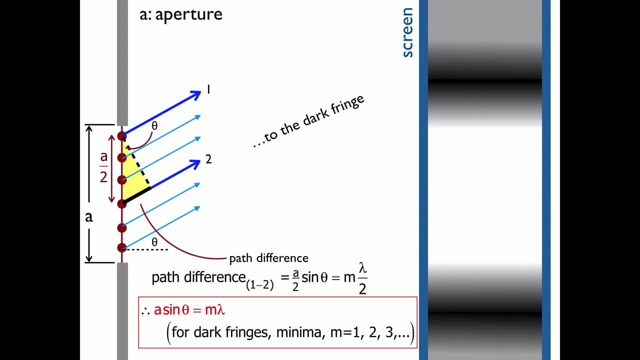 or the minima or destructive interference, And that uses our order numbers of 1,, 2,, 3.. There's no 0 in this one. Now, the same analysis works for all particles, So I'm going to look at the top little particle. 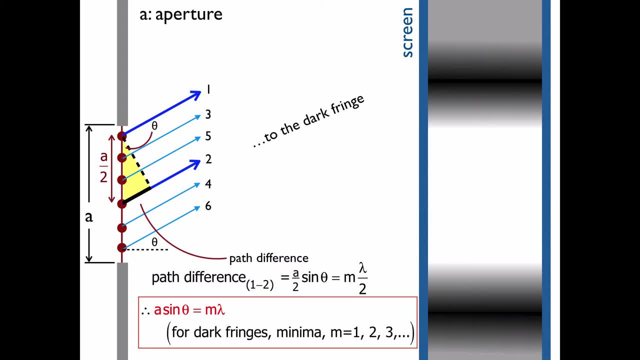 It's the way front. There's 2 long way front, not just the 2 that I've chosen, because if I try 1, like, say, number 3, on the screen, there's another particle somewhere. that's one half a away from number. 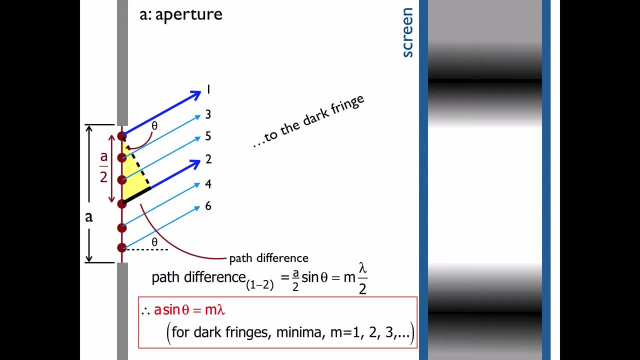 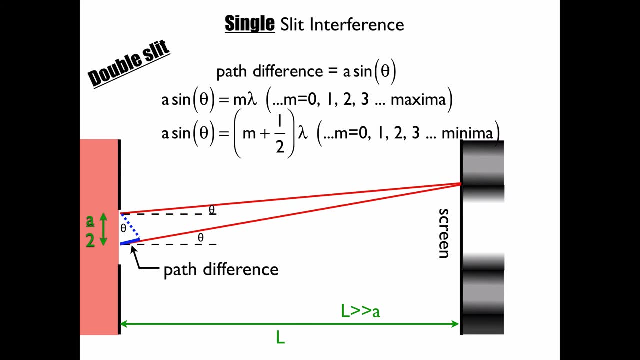 3. That would be number 4.. And then, for number 5, there would be another one that's one half a away, and that would be number 6.. So it works for all particles along this screen. Alright, let's compare this to the double slit. 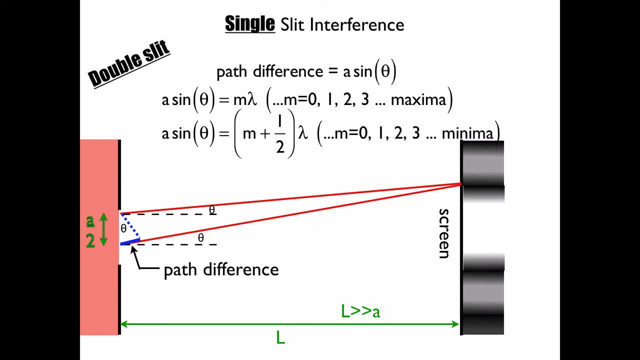 So the single slit sets up something like this, with the path difference going to the single dark slot over there, And this is what we had for the double slit. look at it for the single slit, For the single slit. what's different is that I'm not going to. 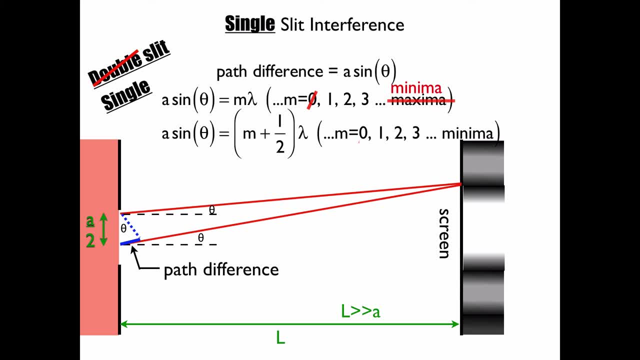 have a zeroth order and instead of a maxima it's a minima. I'm going to look at the other one again. no zeroth order. Instead of a minima, it's maxima. So the equation's reversed, Okay.